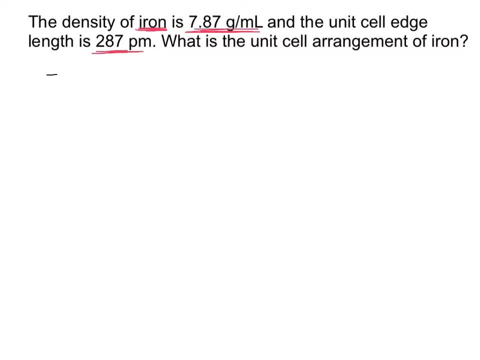 molar mass. So I'm going to start with my given information. I'm going to start with the 7.87 grams per centimeter cubed. Notice, I changed that milliliters, sorry- immediately to grams per one centimeter cubed. My reason for doing that is: 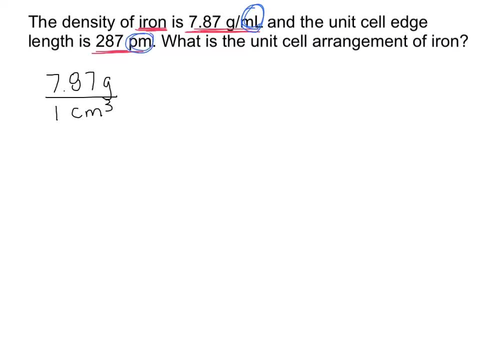 because my volume unit here is going to have to eventually match that volume unit there, And so as I go along, I'm going to keep working everything towards centimeters cubed in my problem. So once I've got that, I'm going to start doing some. 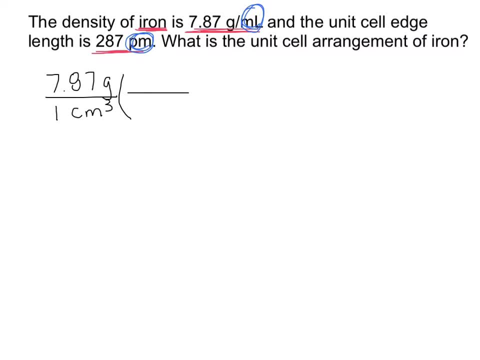 conversions, and the first conversion I'm going to do is get me from grams to moles, because grams to moles will eventually get me from moles to atoms. And so I know, in one mole there's 55.85 grams of iron, and in one mole there's 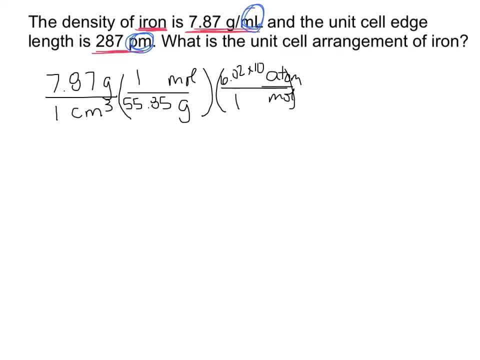 Avogadro's number: 6.02 times 10 to the 23rd atoms, And when you punch this into your calculator you get 8.. I'm not going to round, I'm going to leave a whole bunch of numbers here: 2,, 9 times 10 to the 22nd. My units are atoms per centimeter, cubed at this: 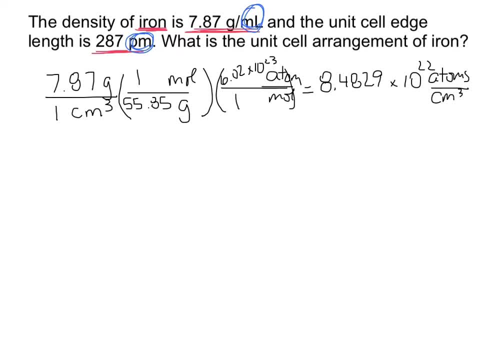 point, And so what I'm going to do next is take my other piece of given information, my 287 picometers for my length of this side, And I'm going to work my way to a volume in centimeters cubed. So my picometers to centimeter conversion, if you don't know that one. 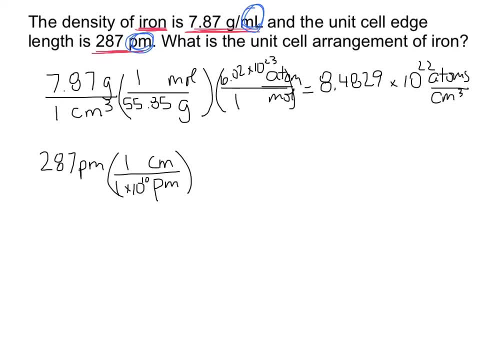 it's 1 times 10 to the 10th picometers in 1 centimeter, And so I'm going to then convert this. Oh wait, I'm sorry, Let me back up a second here. I'm not going to do a conversion here. 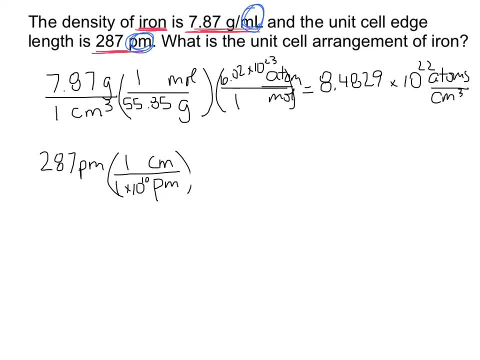 I'm going to get my number And at that point I'm going to have. if I punch that in, I get 2.87, of course times 10 to the negative 8th, And that's in centimeters. 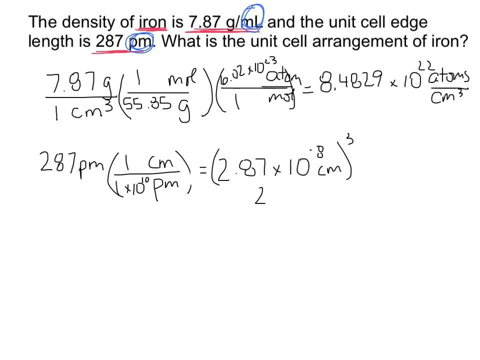 And what I'm going to do is cube this to get me 2.364 times 10 to the negative 23rd, And this is centimeters, cubed This, of course. here is my volume of 8. I'm just going to label it. volume of 1 cell. 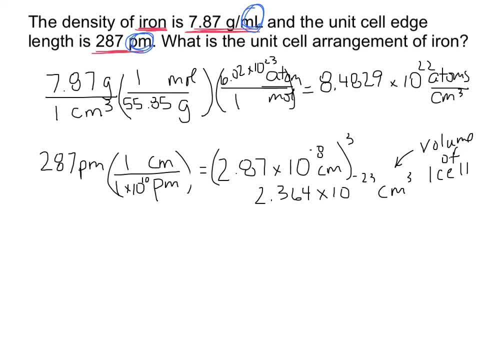 Now, if I know that this is the volume of 1 cell here, and I know that there are this many atoms per centimeter cubed, then I can very easily figure out how many atoms per cell there is by setting up a little proportion. 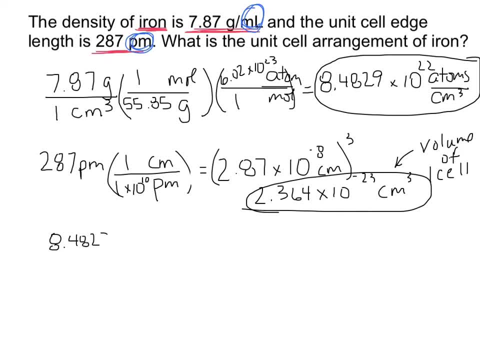 So if I have 8.4829 times 10 to the 22nd atoms- I'm just going to make it 18, per 1 centimeter cubed, then I have X number of atoms per 2.364 times 10 to the negative 23rd centimeters cubed. 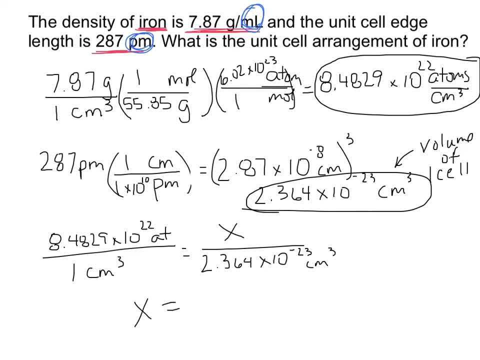 And when I solve for that, I end up with 2 atoms. 2 atoms, tells me. therefore it is a body centered Arrangement, Because body centered, I know, has a total of 2 atoms per unit cell. So you can see none of this math is terribly difficult. 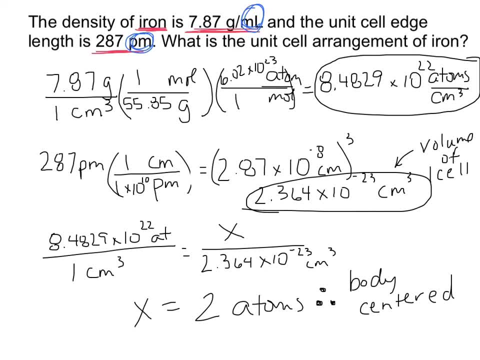 It's a matter of understanding the conversions and it's a matter of using what you have to get to what you need. A little bit of practice makes these a whole lot easier, because you can kind of work your way through some of the different given information. 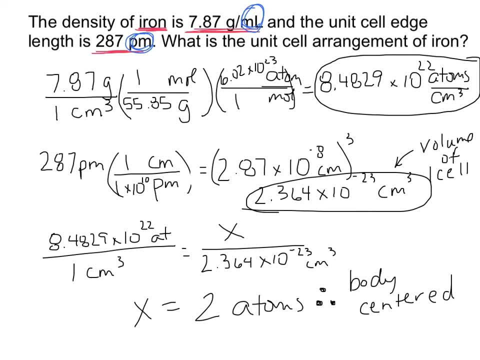 and what you can use to get with that information. If you start, for example, knowing that it's body centered, then you know this, that there's 2 atoms per unit cell. If they start you with the side, we can get to a volume. 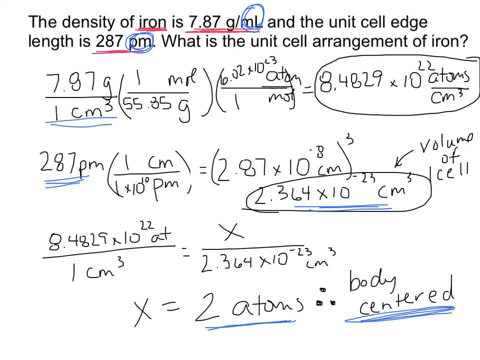 If they start you with a density, we can work our way to an atoms per centimeter cubed. If they don't have a density, but they tell you what element you're working with or what compound you have, a molar mass.